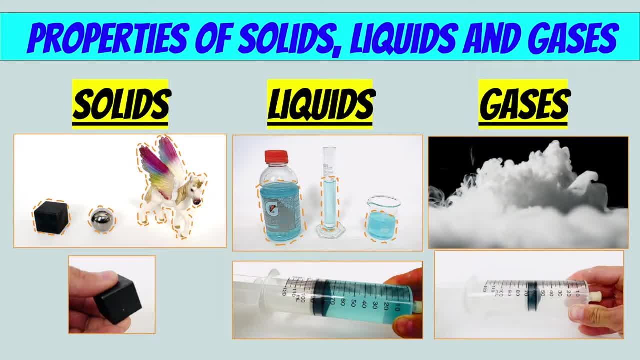 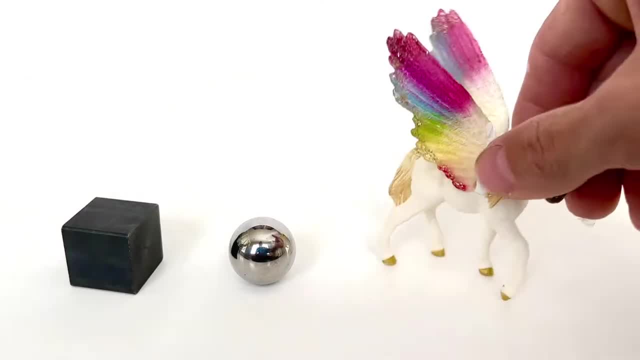 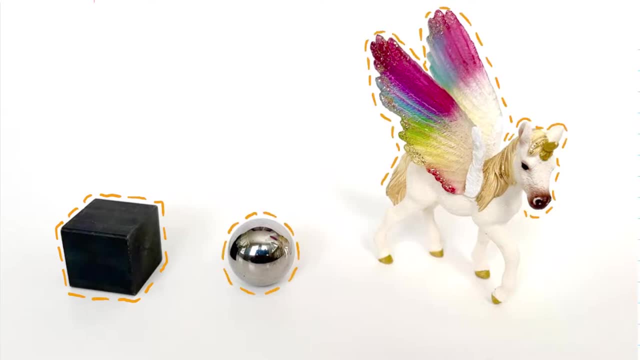 In this video, we're going to take a look at the properties of solids, liquids and gases. Let's start by taking a look at some solids Now. the first thing you'll notice about a solid is that they hold their shape. Whether it's a cube sphere or even an alicorn, they have a definite shape, which means they hold their shape. 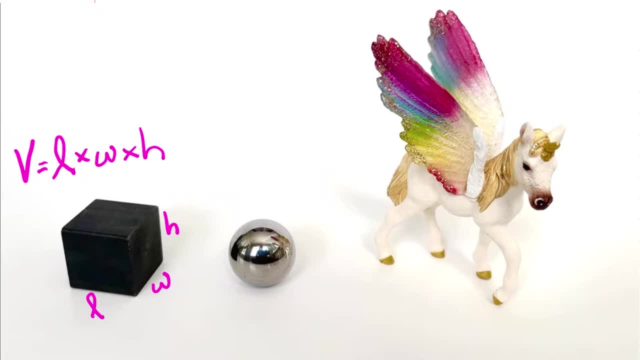 Since solids hold their shape, they also have a definite volume, which is a volume that doesn't change. With regular shapes, like a cube or a sphere, you can use a formula to find the volume, Whereas something that's irregular, like an alicorn, you'd have to find the volume through water displacement. 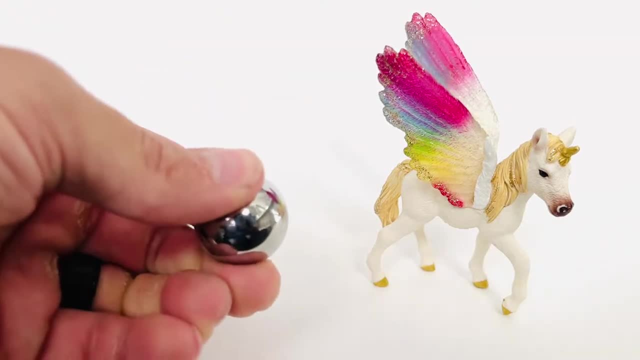 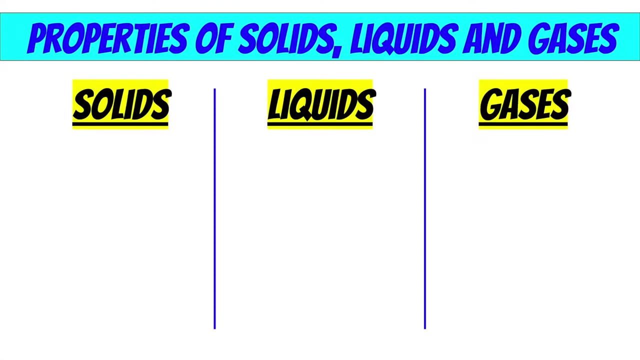 One final property of a solid is they are not easily compressible. So if you try to squish a solid, it generally tries to hold its shape. So, to summarize, solids have a definite shape, definite volume and are not easily compressible. 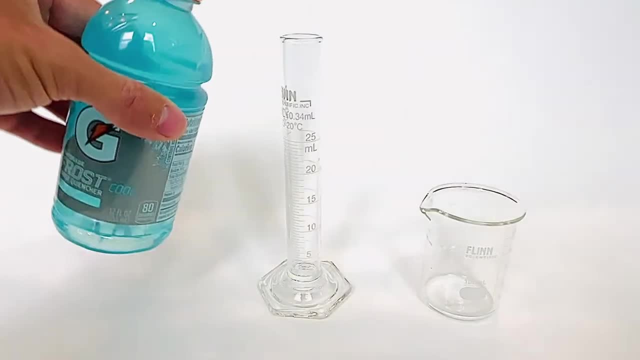 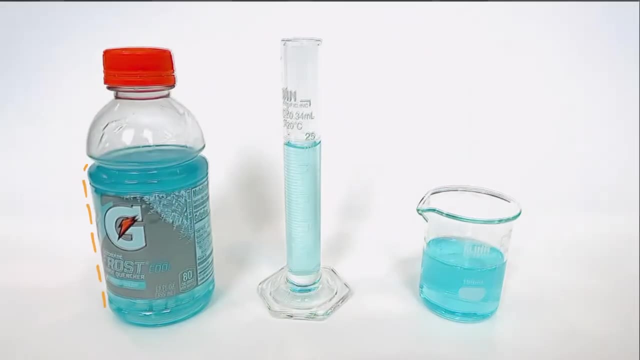 Let's go ahead and take a look. The first thing is: let's look at the shape of a liquid. Now, if we pour a liquid into other containers, we'll notice that it's no longer the same shape as shown by the outline here. 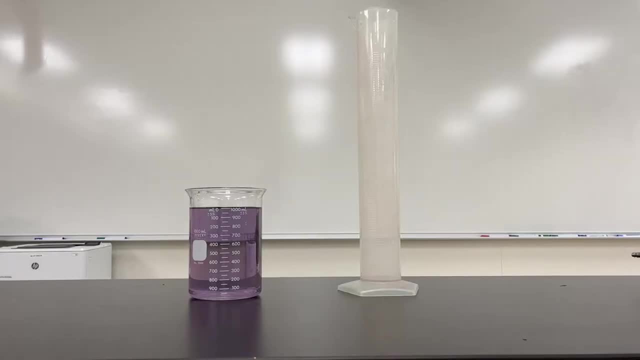 Now let's take a look at a liquid to see if its volume changes when we change its shape. Here we'll start with a thousand milliliters of a liquid and we'll change its shape by putting it in a large graduated cylinder and see what the volume reads afterwards. 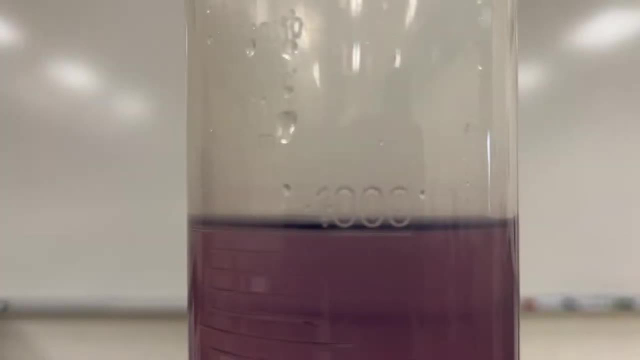 So after we change its shape, you can see that the liquid is still at a thousand milliliters. Therefore its volume did not change, so it has a definite volume. Now let's take a look at a liquid to see if it's compressible. 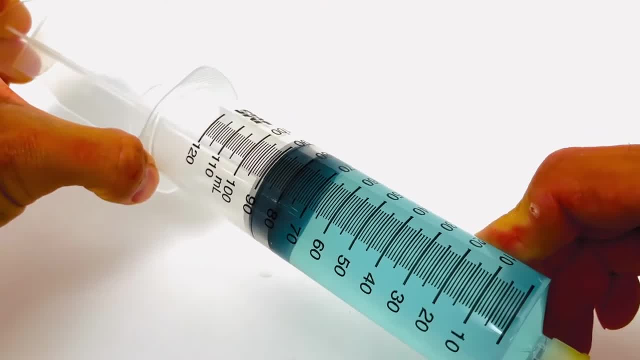 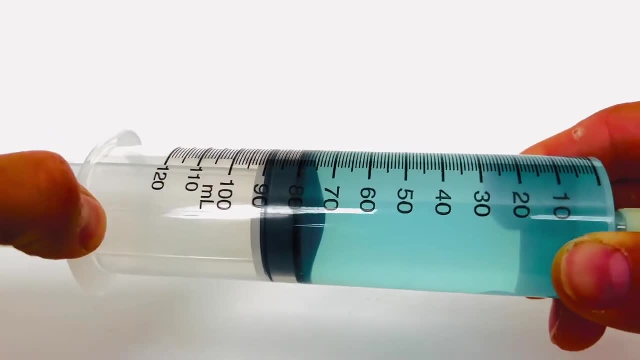 We have the syringe here and inside of it we have a liquid and I'm going to try to push on it to compress it into a smaller volume. So here I am squeezing it, pushing on it, and it's at 80 milliliters and it doesn't seem to be changing. 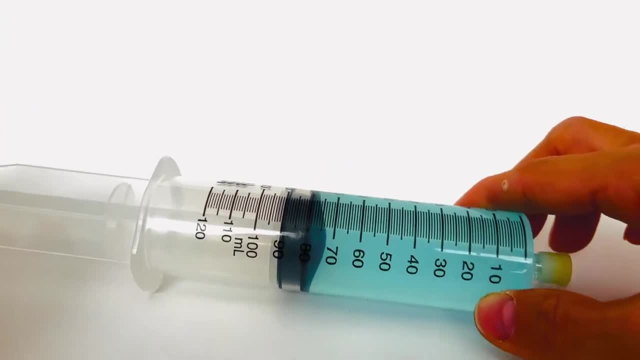 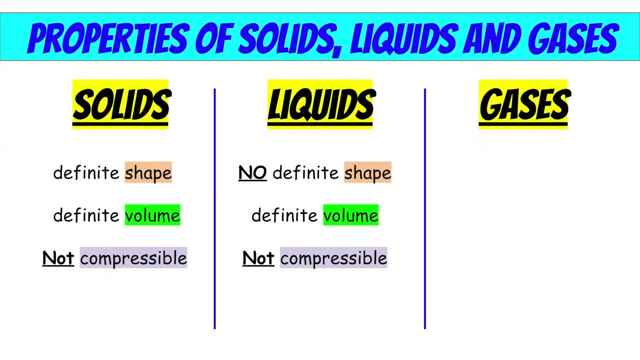 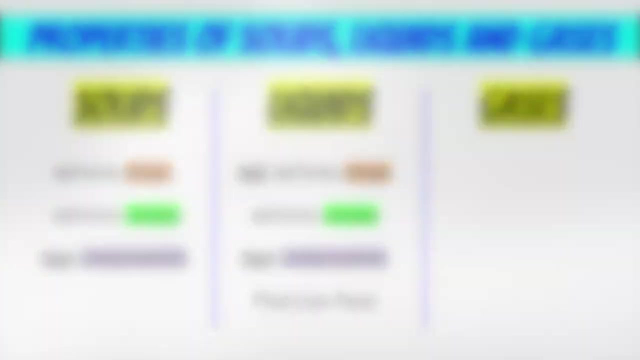 This demonstrates that liquids are not easily compressible. So, to summarize, liquids have no definite shape, have a definite volume, are not easily compressible and one last property is that they are fluid, since they can flow. Finally, let's move on to gases.